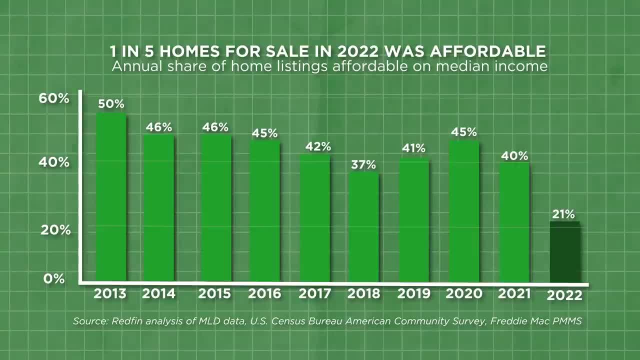 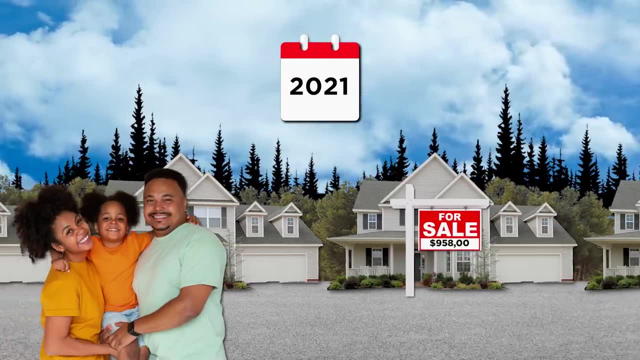 only 21% of homes that went on sale in 2022 were considered affordable. That's down from 60% of homes that went on sale in 2021. That means in just one year, two-thirds of all affordable housing became too expensive for the average. 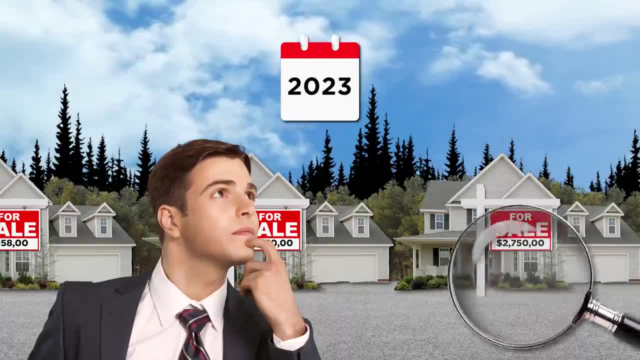 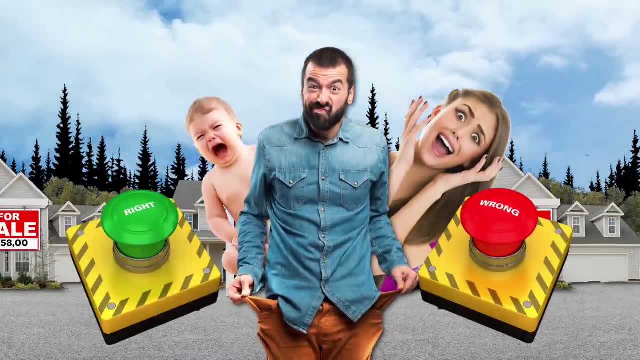 American. The team conducting this survey concluded that housing affordability is at its lowest point in history. But what's the endgame here? If people can't afford a home, then house prices can't go up anymore, Right Wrong? I don't want to make another one of those stupid finfluencer videos about how the housing market 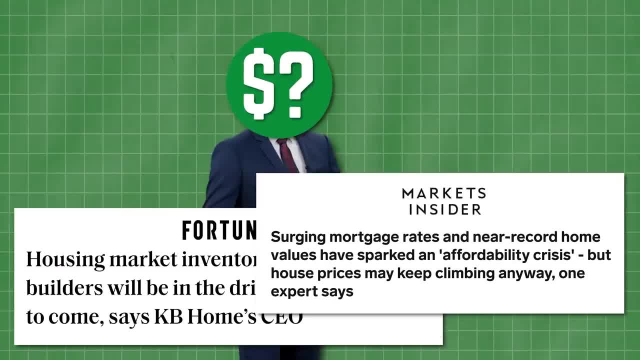 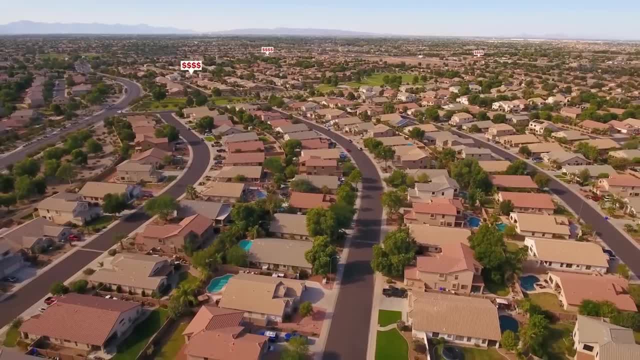 is going to crash in 3.5 days, but there are three reasons why it could get a lot worse before it gets better. The first reason is that houses do not need to be affordable for you to buy one If you think that can't make sense. 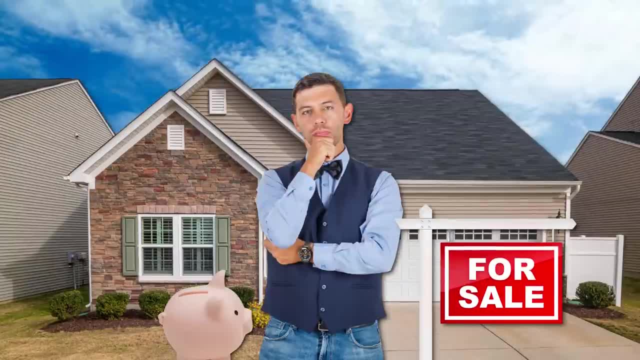 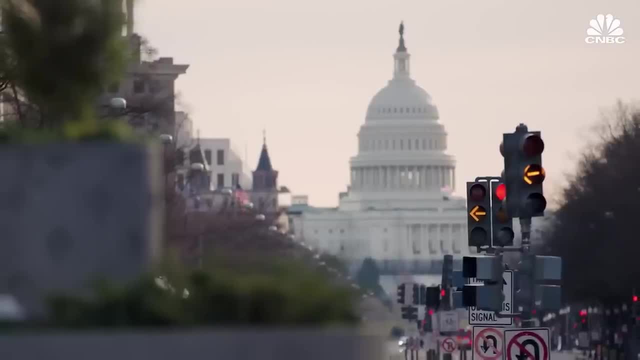 there is an entire industry working to make it true. You don't save money to buy a house, you save money for a down payment. The housing costs are completely out of line with wages. Wages have not cupped up with house prices, but a 20% down payment only grows at one-fifth the 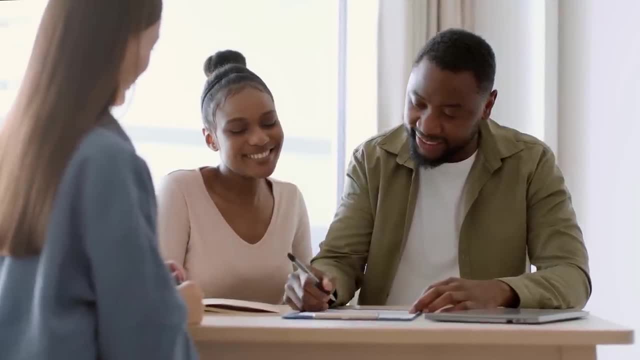 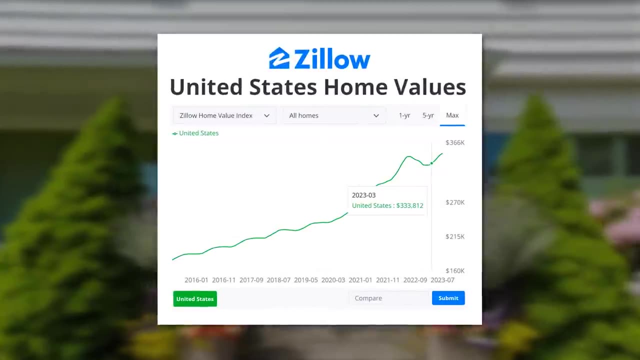 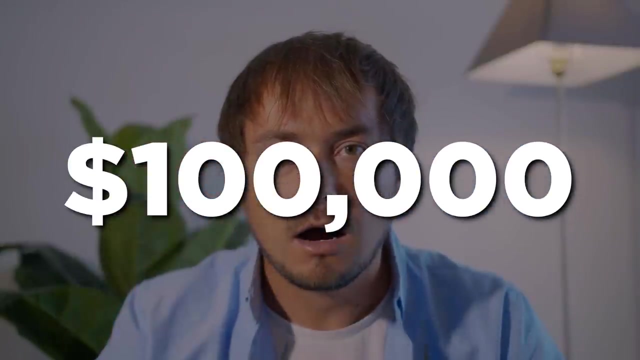 rate in absolute terms, so people are still able to get into the market. According to Zillow, the average home sold in America in 2020 traded for $230,000,. at the start of 2023, the average home price was $330,000, a jump of $100,000 in less than three. 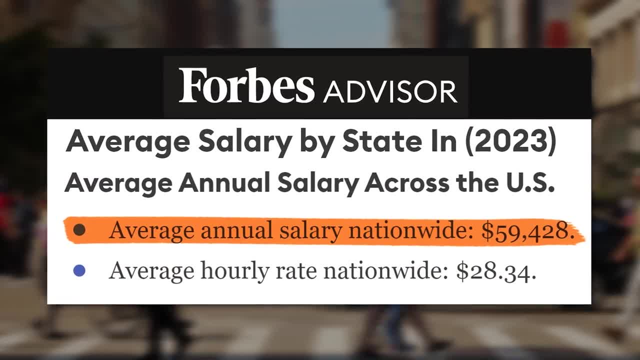 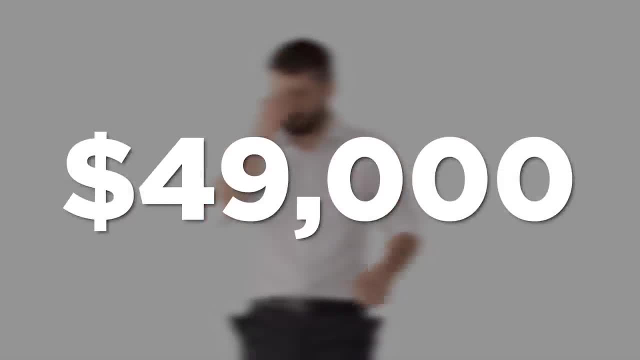 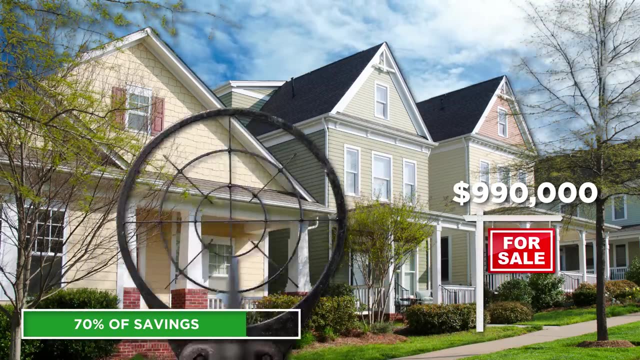 years. According to Forbes, the average American makes a salary of $59,000 before tax. after federal tax in FICA, that leaves them with a take home of $49,000.. If this average person saved a ridiculous 70% of their take home pay to buy a house, they would be just as far away from their 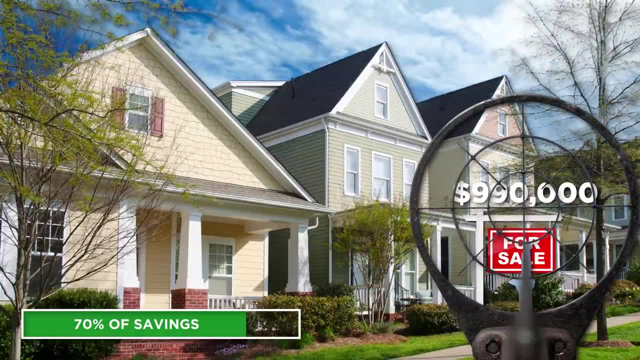 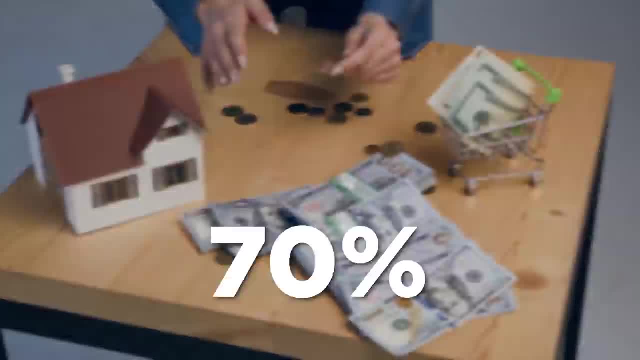 goal after three years because the price of the average house grew just as fast as their savings. The average home earns as much as the average person, but most people only save for a down payment, so 70% becomes 14%, or 7% if it's a dual-income household where the other partner 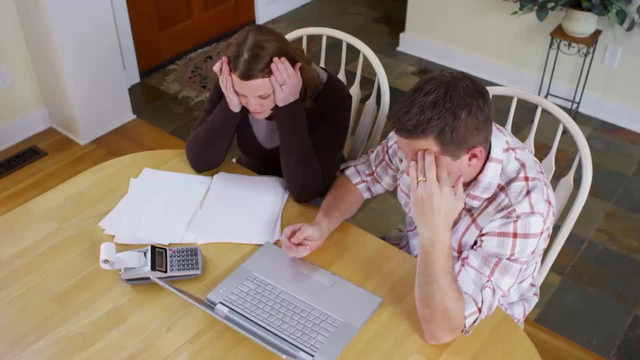 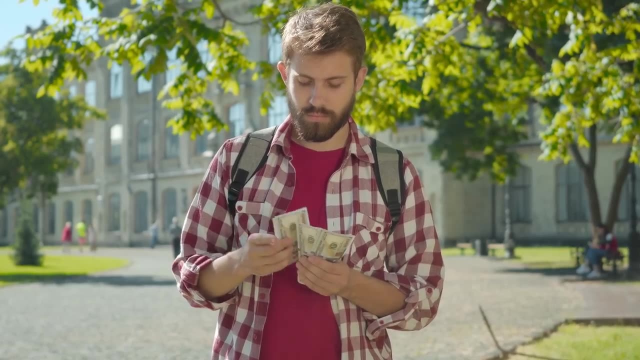 also earns the average salary, That's still a major savings commitment when 57% of Americans can't afford a $1,000 payment without taking on debt. 14% of your take home pay should be more manageable than 70%. but remember, this is only how much you would need to save just to keep up. with price increases. This doesn't actually do anything for you if you don't save as much as you would if you were to buy a home. Lenders and banks with a vested interest in real estate assets across the country know that it is still hard for most families, who also need to pay for. 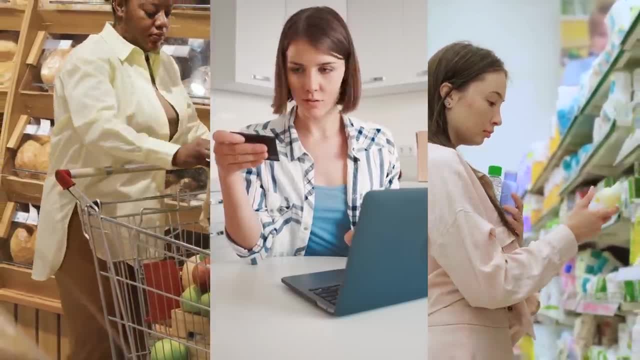 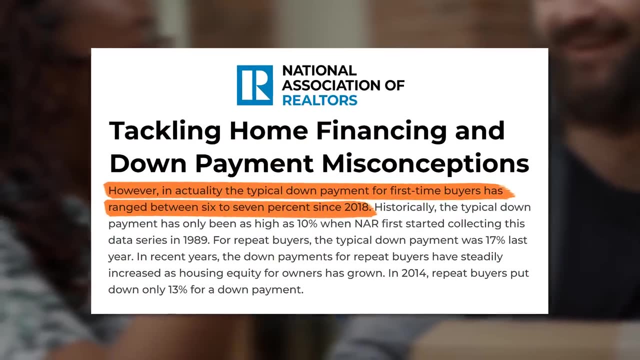 food, rent and other essentials that are outpacing wages. so they have moved the goalposts. A report by the National Association of Realtors found that the average down payment for a first time home buyer was just 7%, and the average down payment for a repeat purchaser that has had time. 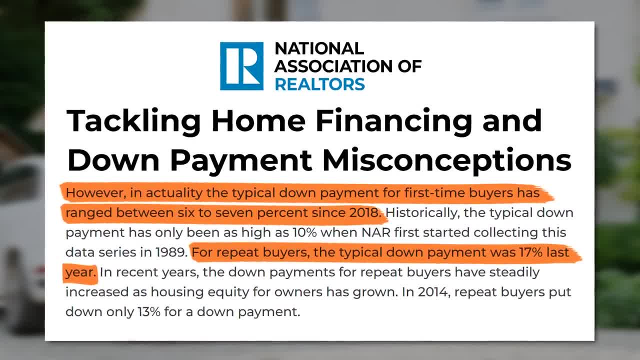 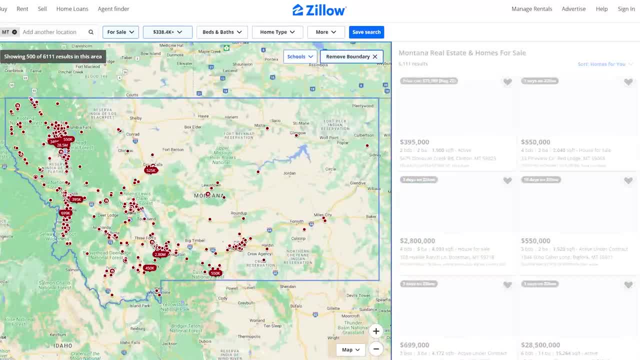 to build equity in their previous home was only 17%. If you only need to put a tiny deposit down, the house prices can increase to many multiples of your income before it becomes impossible to buy a house. If you only need to save for a 7% down payment, then just a 10% savings rate over. 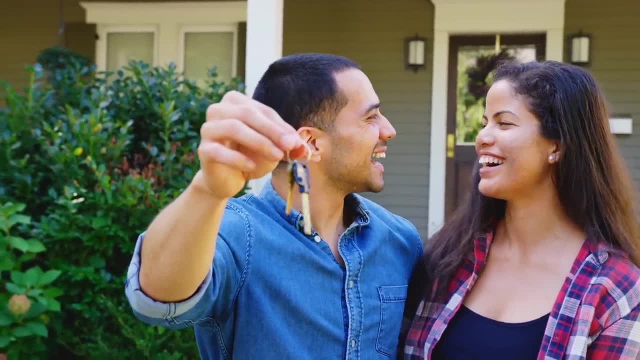 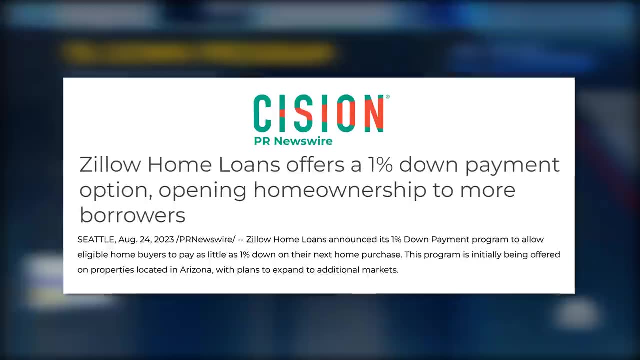 three years from an average wage would get you into an average house. You would be more disciplined than the average American, but it's not impossible with some sacrifice. If that's still too hard for you, then Zillow recently announced that they would be trialing a 1% down payment loan product. 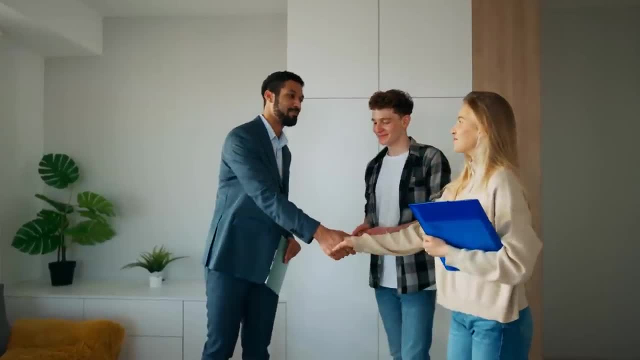 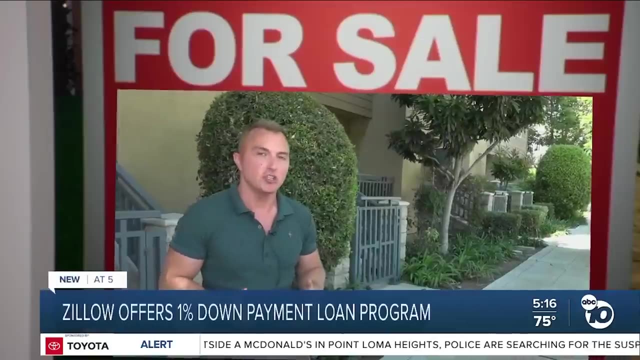 to help people that couldn't save any money make the biggest financial commitment of their lives. Here's how it works: The buyer pays a down payment of 1% and then Zillow makes an additional contribution of 2% at closing. That is a grant and doesn't need to be paid back. 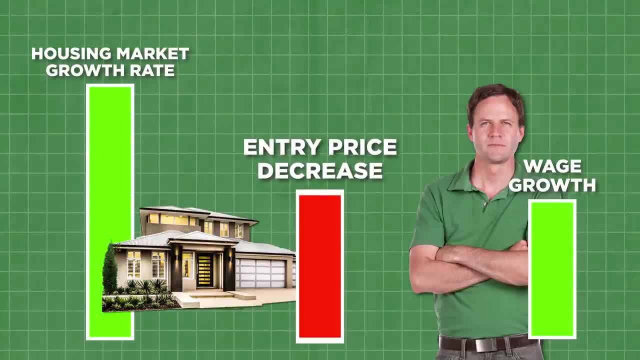 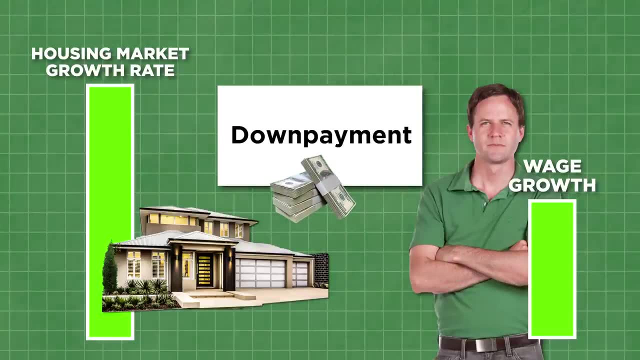 So, even though houses are making more money than you are, the price of entry is being reduced just as fast, But that's only to make the down payment. You still need to make the repayments, and if you can't put 20% down, what hope do you have of making repayments on a house? 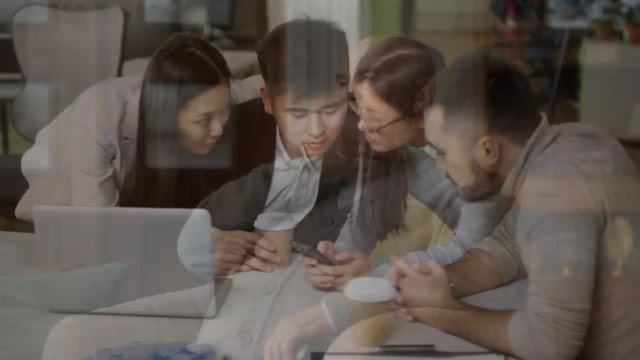 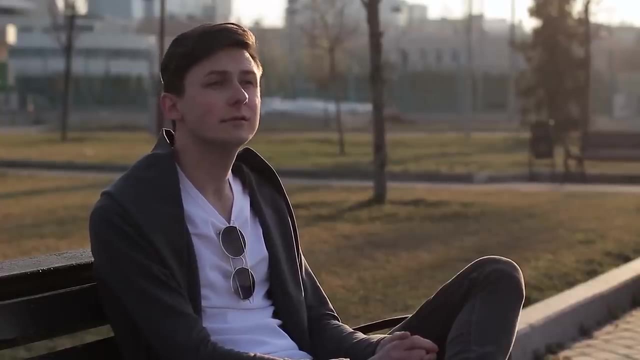 Well, it's time to learn how money works, to find out if the circus really can go on forever. This week's lesson is sponsored by Trade Coffee. Now, I know that this may not come as a surprise to most of you, but my team and I need a lot of coffee to keep making content on how money works. 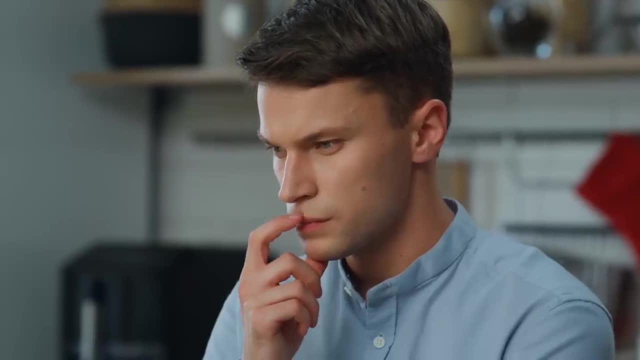 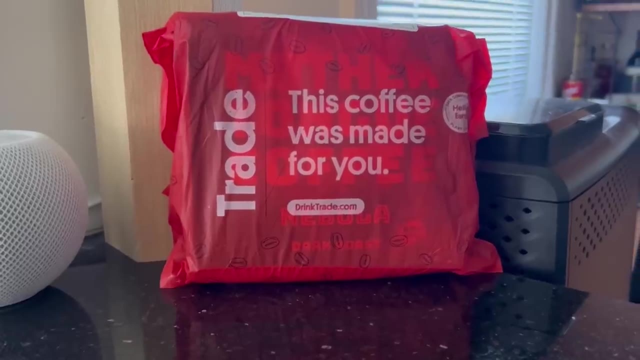 how history works and compounded daily. But I've been sticking with the same coffee for a while. I mostly just drink the same boring coffee just to get me going. But now, since I've been using Trade Coffee, my old coffee seems like it's just gross and just not tasteful. 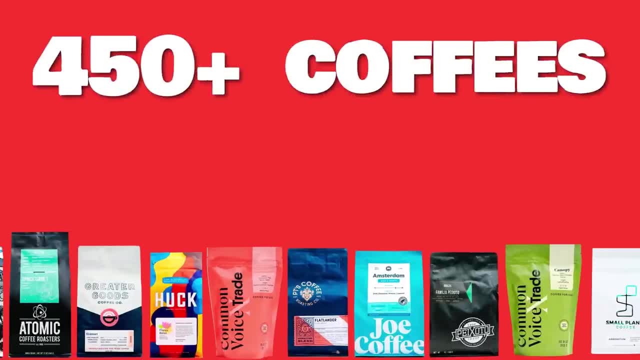 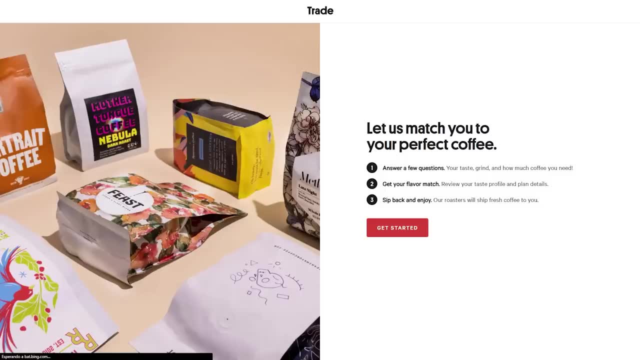 Trade Coffee has made coffee exciting again, connecting me with over 450 coffees from over 55 roasters, including dark roasts, espresso blends and rare roasts. Their matching algorithm curates the perfect coffee match for you based on your taste. 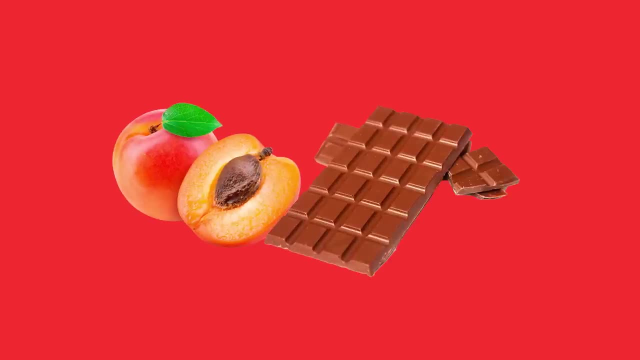 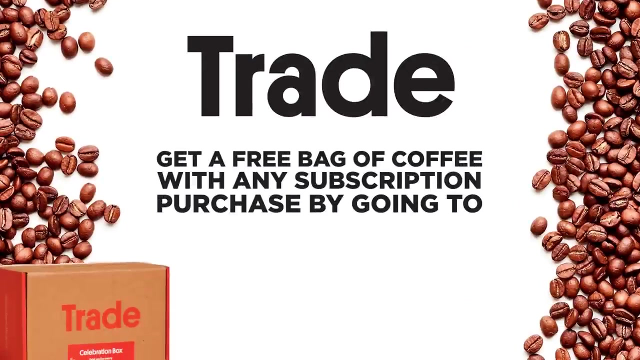 preferences. For example, I prefer fruity with notes of chocolate. so Trade matched me with Sightglass Organic Toca Tea, and it was absolutely delicious. Get a free bag of coffee with any subscription purchased by going to drinktradecom forward. slash howmoneyworks With free shipping. 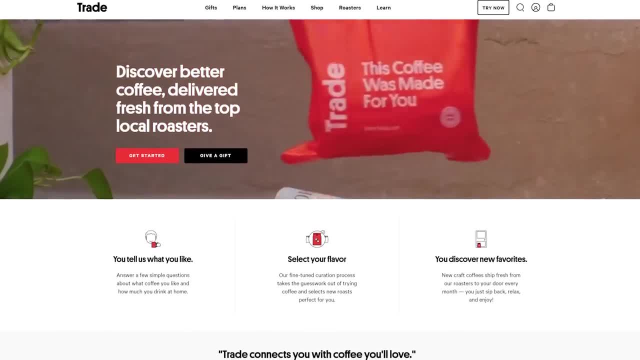 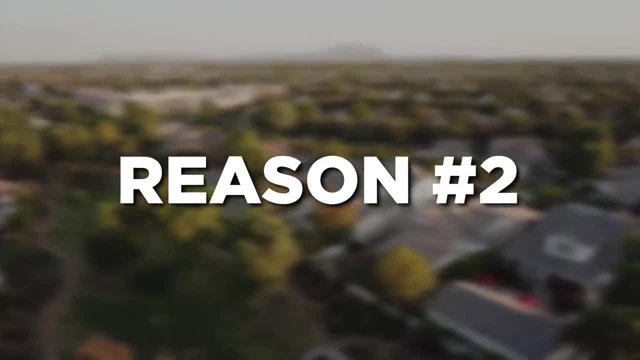 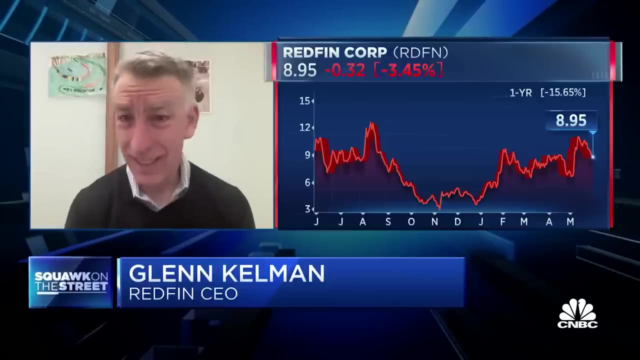 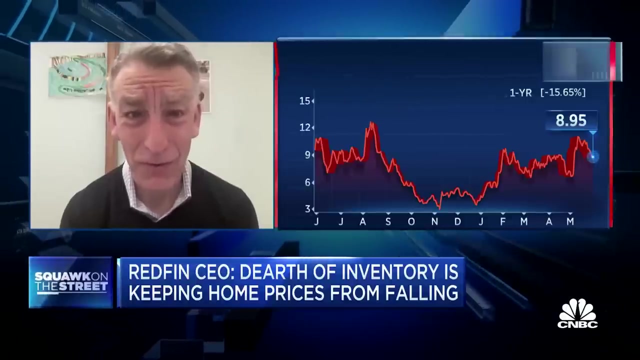 customizable plans and anytime cancellation. Trade is making it easier to discover better coffee. The second way that houses can keep on getting more expensive, even when nobody can afford to buy them, is because nobody is selling them. Home sales in America are at their lowest level in a decade, despite population growth, According 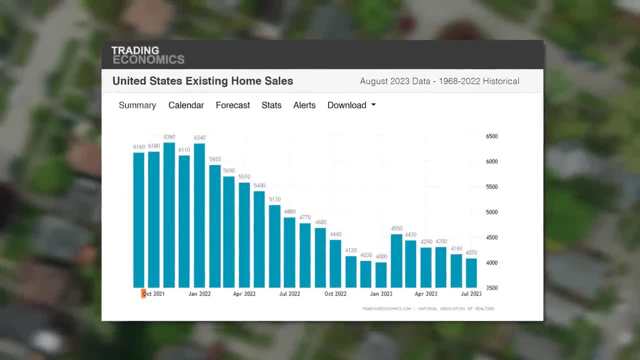 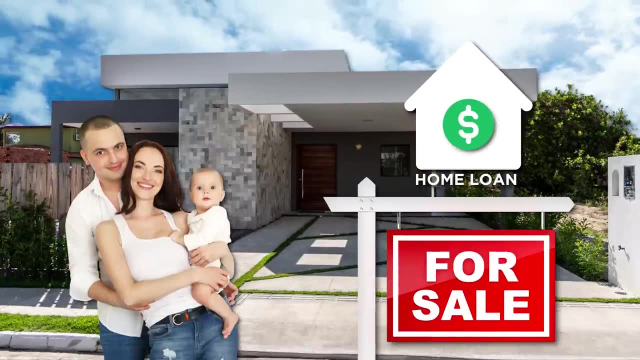 to data from the National Association of Realtors, six million homes were sold in 2021, but now only four million homes are selling at an annualized rate. Potential sellers with a home loan don't want to sell because the rental market is even more unaffordable and if they move into a new. 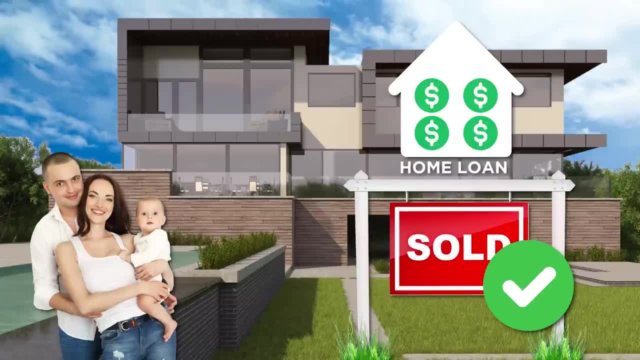 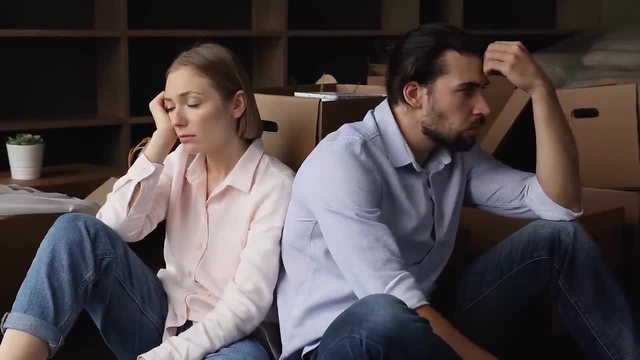 home, they will get a new home loan that has a much higher rate than what they are paying currently. Many people already moved during COVID and another move so quickly would be too disruptive on their social and family lives, in addition to the significant interest expense of new home loans. 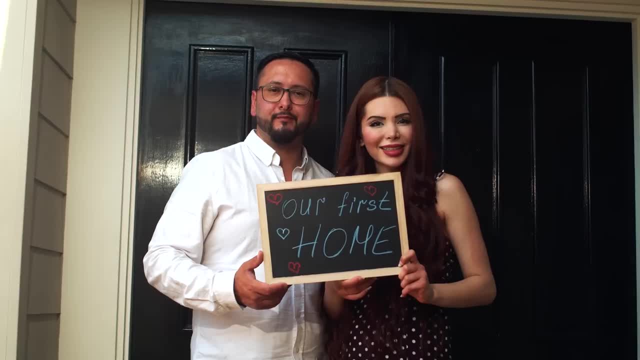 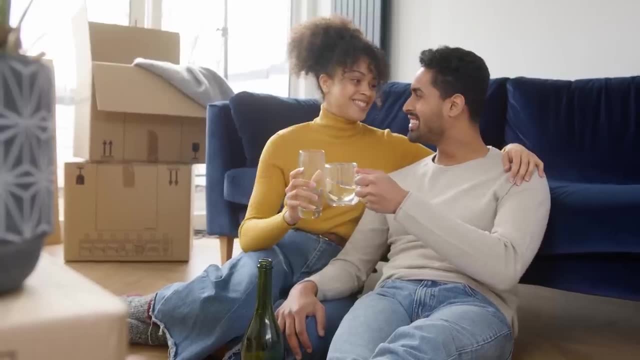 The average homeowner spends 13.2 years in their home. After a flurry of home buying activity in the last three years, more Americans than ever are just settling into their new home, and they have longer than ever before they consider selling. New buyers are also choosing. 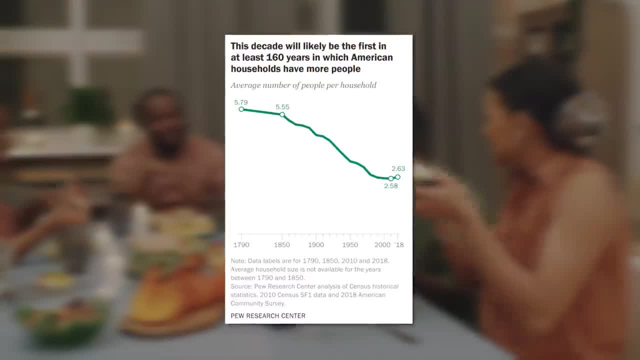 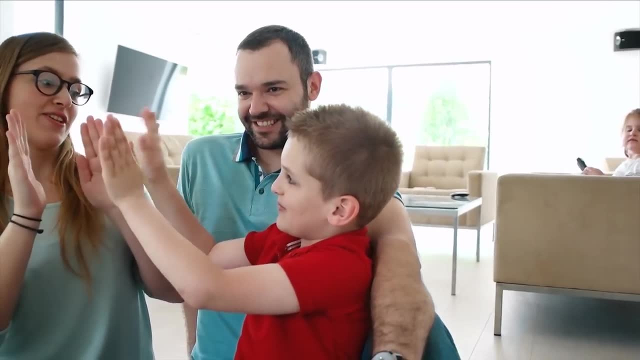 to wait out their purchases until interest rates drop. The average number of people living in a household also increased recently for the first time in 160 years, after a long trend of smaller families and people choosing to move out into their own homes. According to Pew Research that 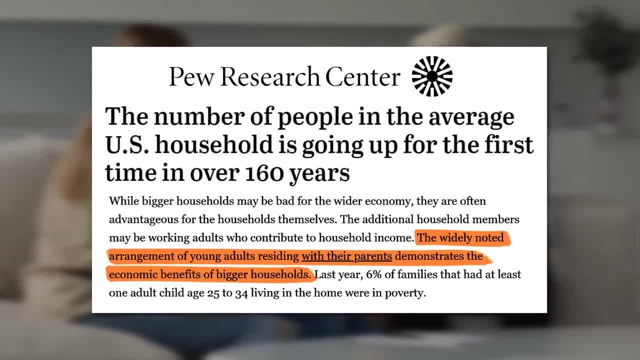 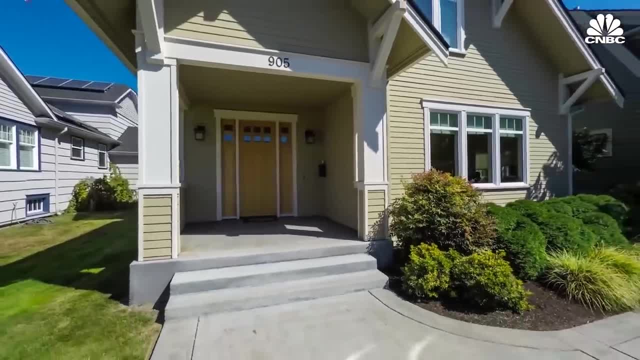 published this report. this was because more younger adults were choosing to, or being forced to, live with their parents for longer to avoid the cost of living with their parents for longer. The average average homeowner is still active, but regular buyers and regular sellers are. choosing to sit out until moving into a new home becomes more affordable. And it's the people who are left that are the third reason. this can keep going on longer than you think. There are three groups still in the game. The first group are all cash buyers that have money. 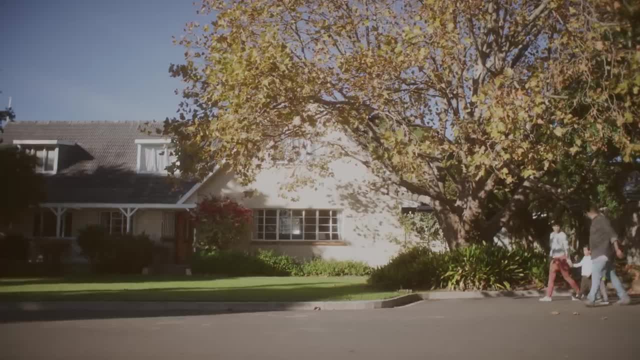 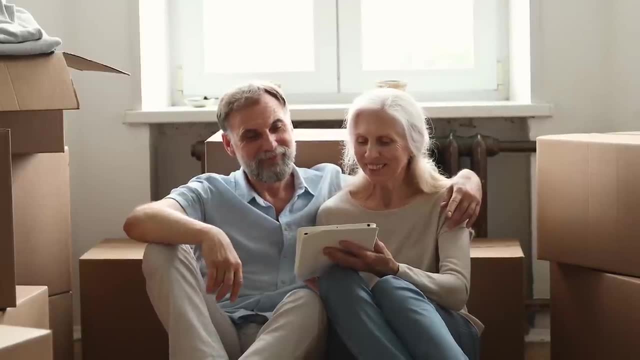 from selling their old home and want to buy a new one. If you were a boomer that purchased their home in the 1970s for three nickels and you now want to downsize, now is an ideal time to buy a new home When prices are higher. the spread between a single-family free-standing home and 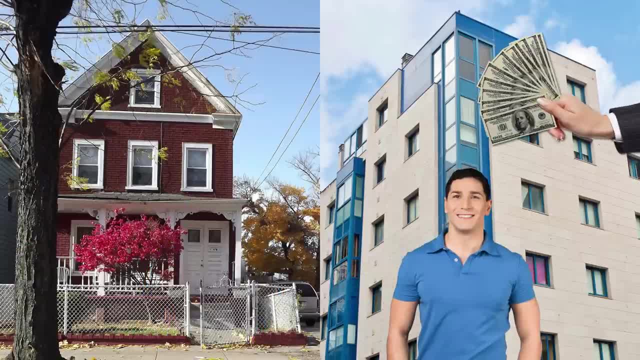 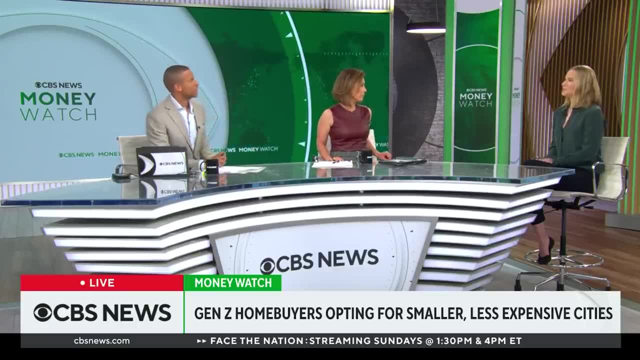 a smaller property is larger, giving you more cash to live off of. The second group are people moving. interstate Unaffordable housing is pushing people out of expensive cities across the country. You would probably prefer to stay in your home city, even if you had a job that you could do from. anywhere. Closeness to friends, family and familiar amenities is why people only live 18 miles from their hometown on average. In defiance of the part-time hedge fund manager and full-time YouTube comedian, Patrick Boyle, I chose to stay in my crappy 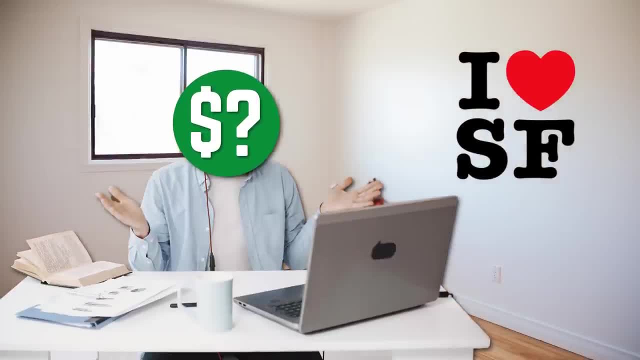 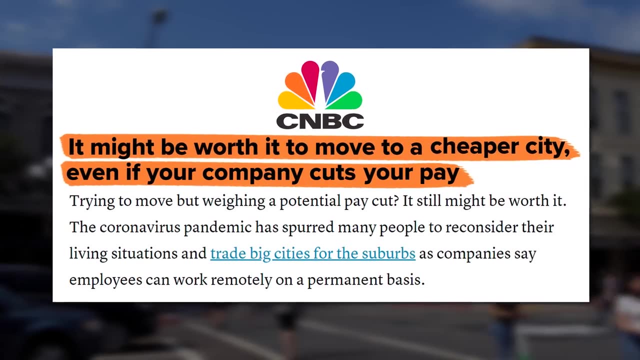 one-bedroom San Francisco apartment because moving is a pain in the ass. But if you are really struggling to afford a high cost of living, you can improve your lifestyle by moving to cheaper cities with lower rents and property prices. If you move from a city like San Francisco, Seattle or New York to any other city in the 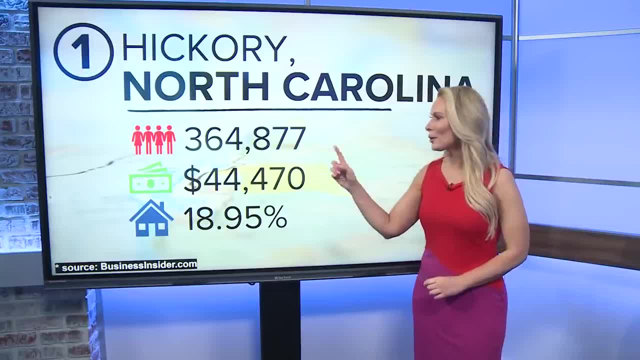 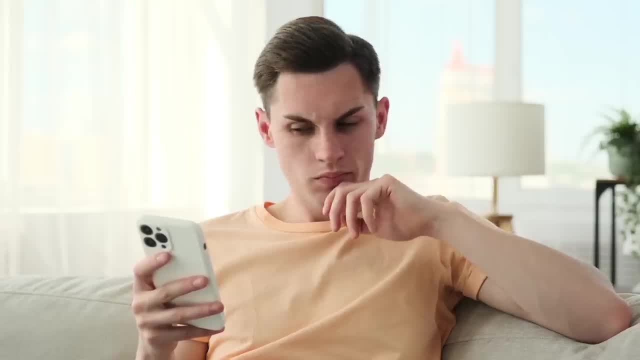 country, you are going to be able to buy a lot more house for the same money. Your higher income from working in these areas will push up local prices And, in the process of avoiding the rising home prices, you have just made it worse And therefore you have more people competing. 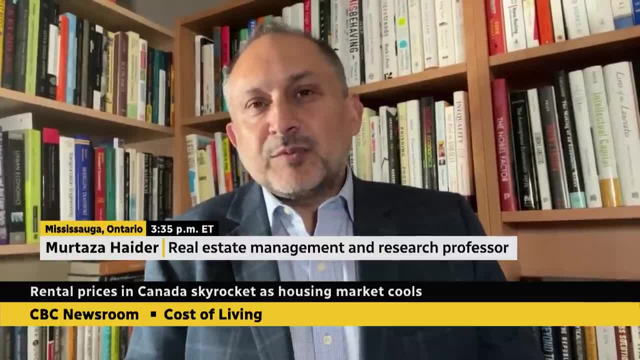 for rental space because the cooling of housing market has kept people longer in rental space And therefore you have more people competing for rental space because the cooling of housing market has kept people longer in rental space. So that is the reason why competition has increased. The supply has been constrained because people 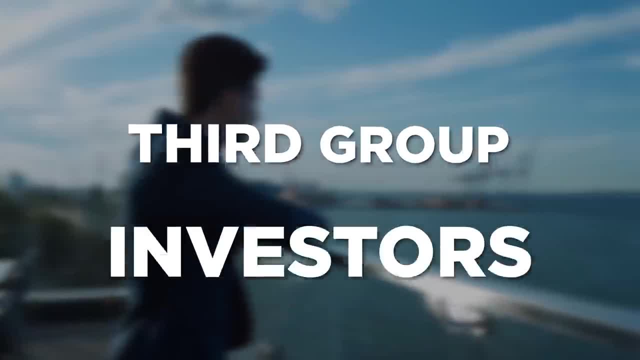 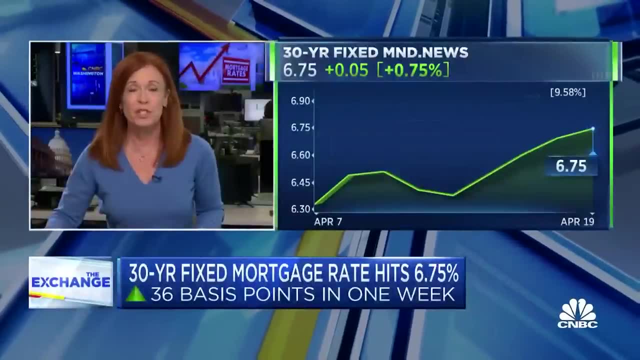 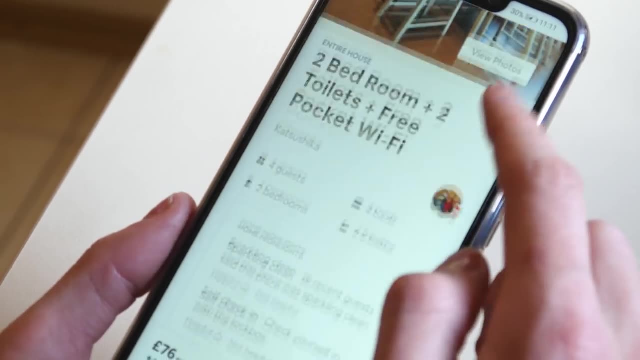 are not moving from rental to owner. The third group are investors. Investors only care about the return on their assets. Prices are high right now and investors using financing to buy property are also paying higher interest rates, But in return, they are charging higher rents to long-term tenants and short-term vacationers, if they 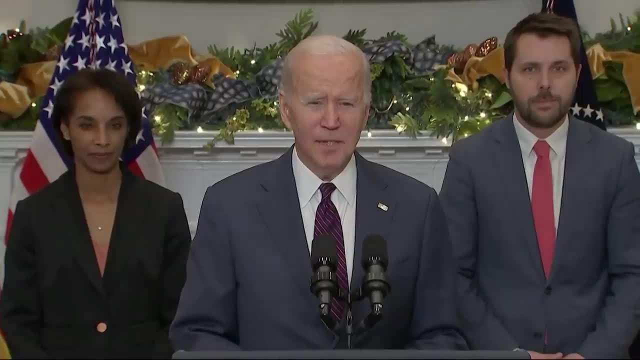 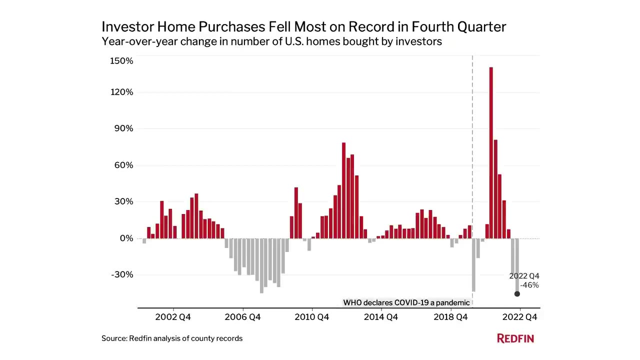 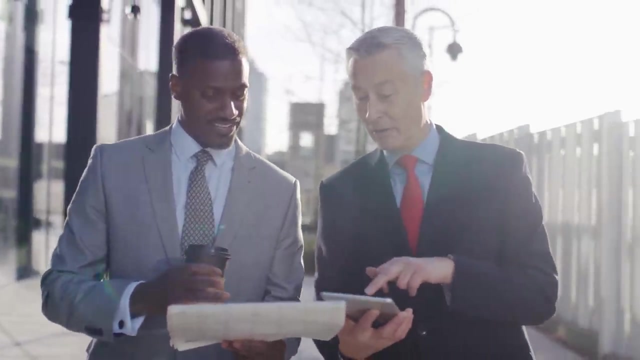 list their properties on sites like Airbnb. Make no mistake: prices are still too high. The largest increase in home buying has come from this group. According to Redfin, year-on-year growth in investment purchases reached 145% in 2022, and institutional investors buying up stock for real estate investment trusts. 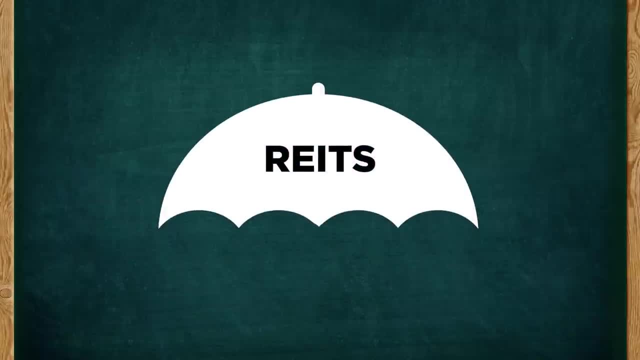 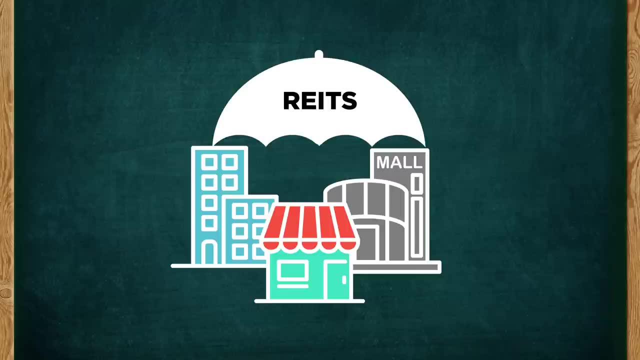 were the fastest-growing group of investors. Real estate investment trusts, or REITs, work like index funds for real estate. They buy a portfolio of properties using money collected from a large group of investors. REITs are sold both over-the-counter through companies like Blackstone. 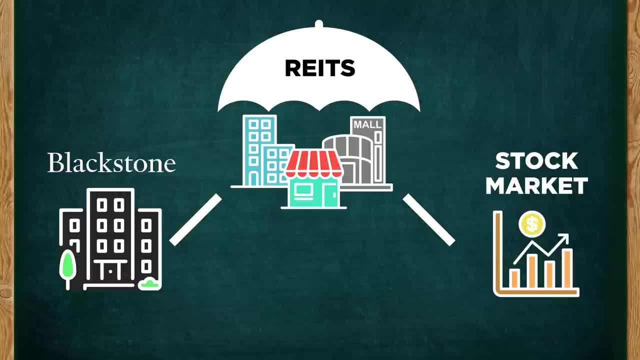 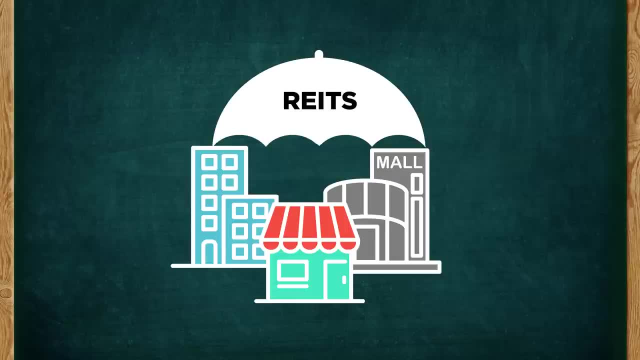 for high-net-worth investors or as exchange-listed securities for average people. REITs used to focus on commercial real estate like shopping malls, hotels, warehouses, office buildings and farmland. The high cost of these properties made them suitable for sharing between multiple investors. Residential REITs have experienced a sharp rise in popularity, though, because people that can't afford to buy a home themselves still want exposure to this market. Some people are putting savings towards the down payment into REITs because they should provide returns consistent. 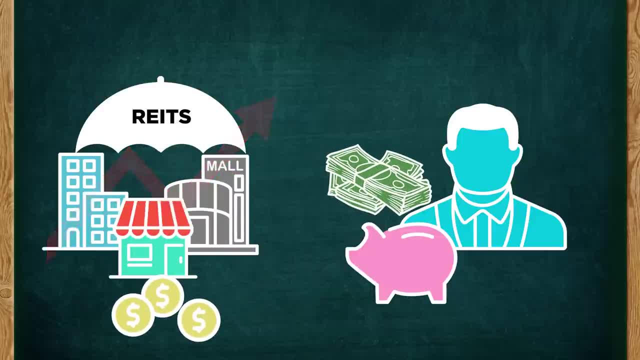 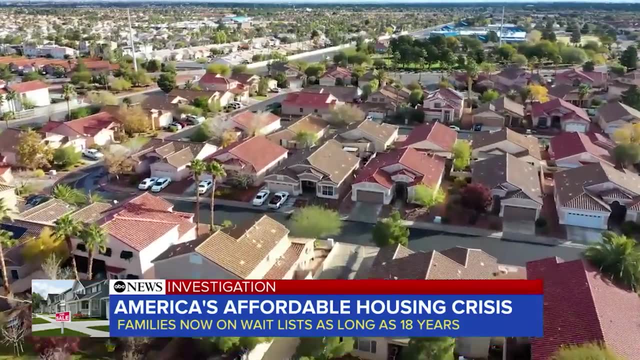 with the residential real estate market so that they can afford to buy a home. Their savings won't be left behind by rising house prices. The popularity of this asset class has been caused by unaffordable housing, and it's also made housing more unaffordable. 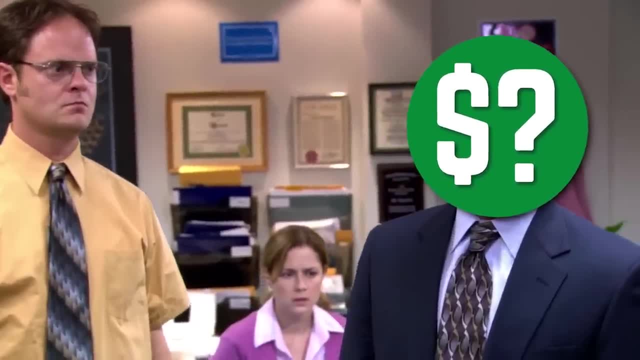 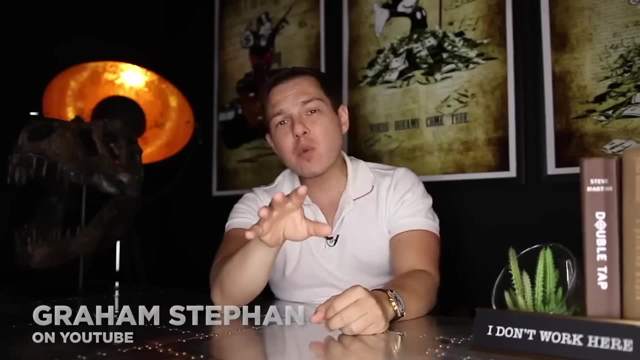 But this can't last forever And, as much as I hate to say it, those stupid fucking finfluencer thumbnails may be right. Things are starting to change. This is why the market is largely resistant to sell-off and why it's still possible for. 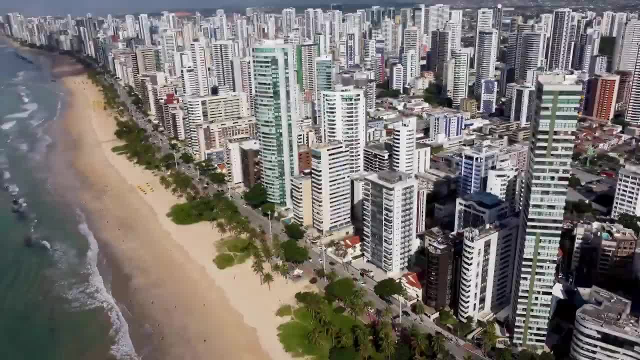 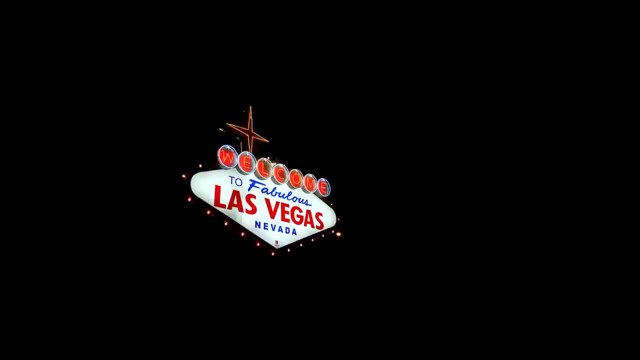 home prices to go even higher, even though it kind of makes no sense. An updated Redfin report has revealed that investor purchases have slowed significantly, and surveys from local agents in cities like Las Vegas, Austin, Miami and Houston revealed that institutional purchases have stopped completely. 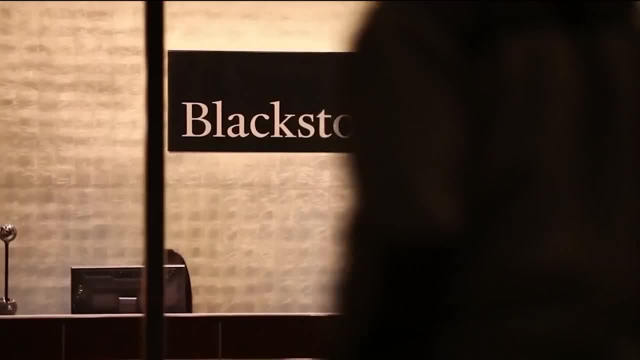 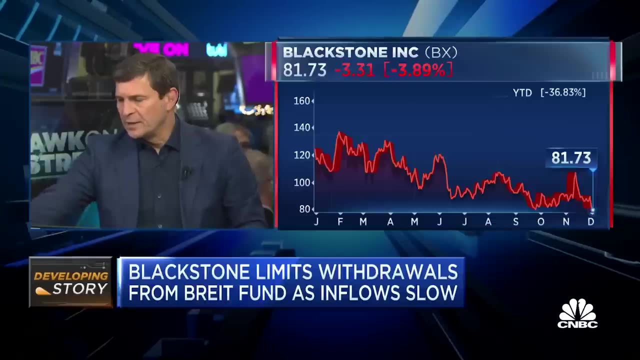 The private equity company Blackstone- not to be confused with the investment index company, Blackrock- had to block investor withdrawals from its $71 billion earlier this year, sparking concerns that the whole system was overvalued. If investors pull their money from these trusts too quickly, the investment managers 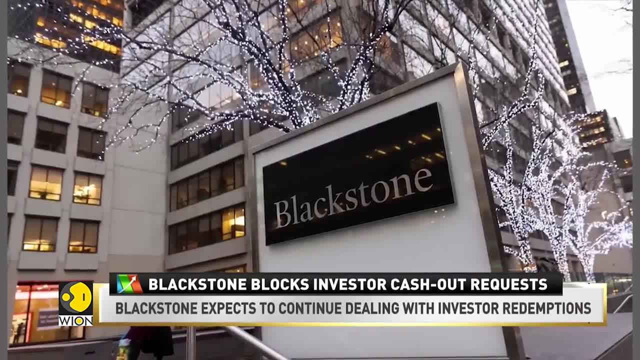 in this case, Blackstone, will be forced to sell one of their properties in their portfolio. Blackrock, which is a company that has been selling property for over a decade, has been accused of overestimating the price of the properties it had in its portfolio. 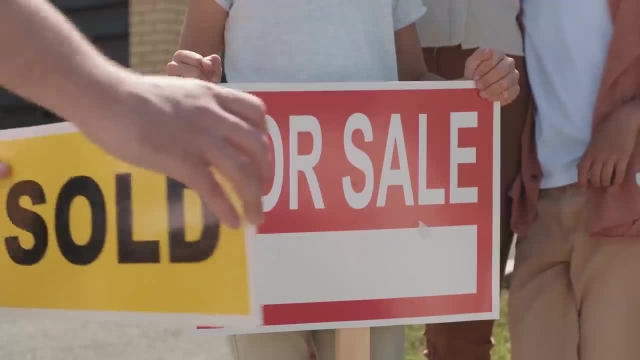 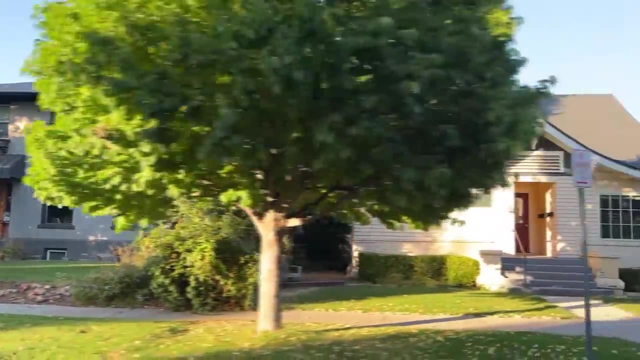 but that's hard to prove until it's forced to sell one of them. But as soon as just one property needs to be sold, all other comparable properties in that trust need to be readjusted to a similar value. A sharp drop in the value of the trust. 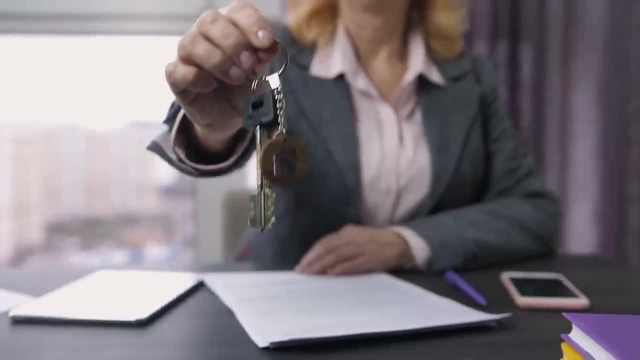 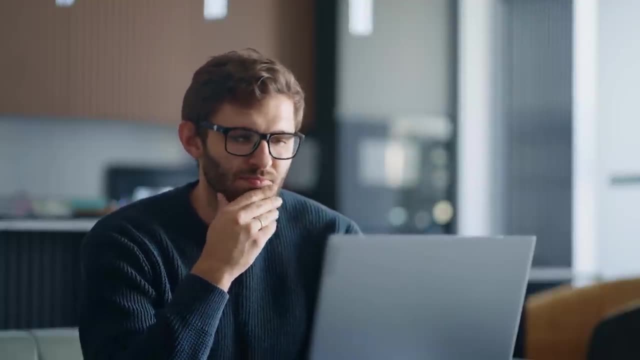 could trigger more investors to withdraw their funds, causing the manager to sell more properties, pushing down prices even further. But don't get your hopes up too much. If you own shares in a REIT, the easiest way for you to liquidate your position would be to sell. your shares to another investor, which doesn't require any cash to be liquidated from the assets themselves. The bonus fourth reason is that wealthy families are just doing a better job of holding onto more properties for themselves. In the past, family wealth struggled to get past.